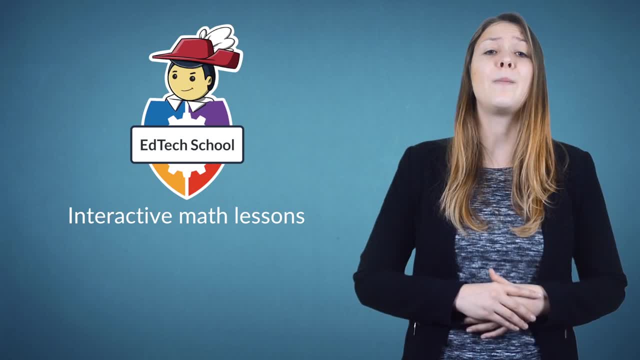 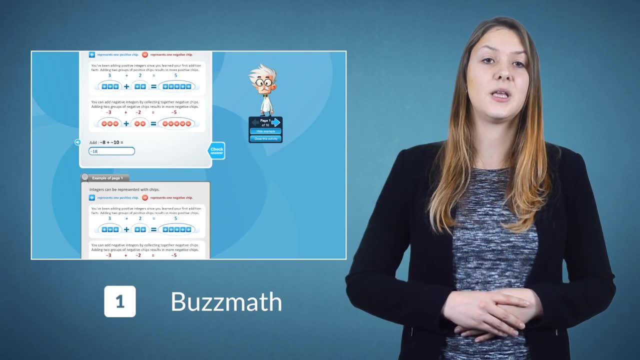 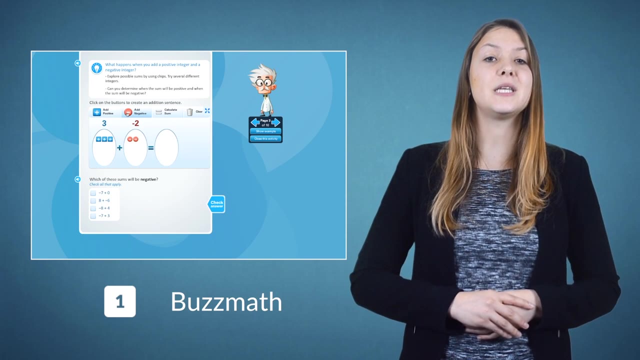 can help students practice math. I sorted out a few amazing apps and websites. The first one is BuzzMath. BuzzMath is a website where your students can practice. Kids are challenged to save BuzzCity from math ignorance. BuzzMath has a list of topics and a core-aligned interactive. 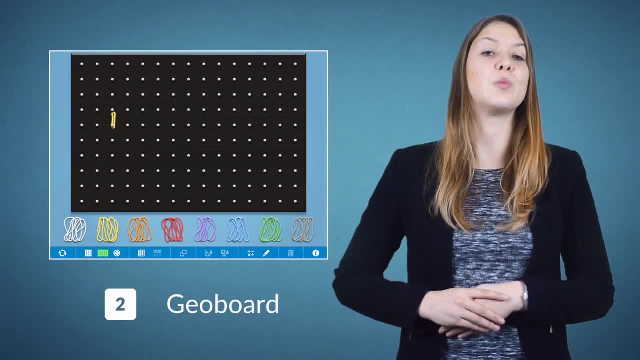 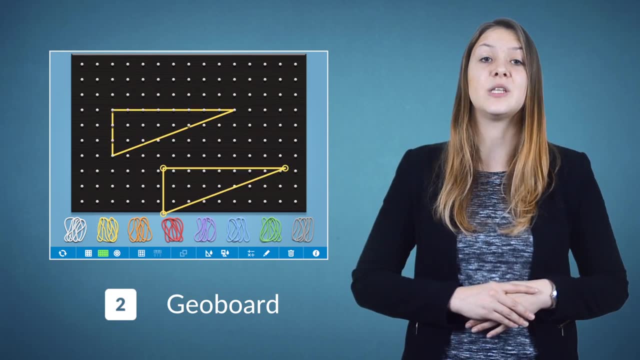 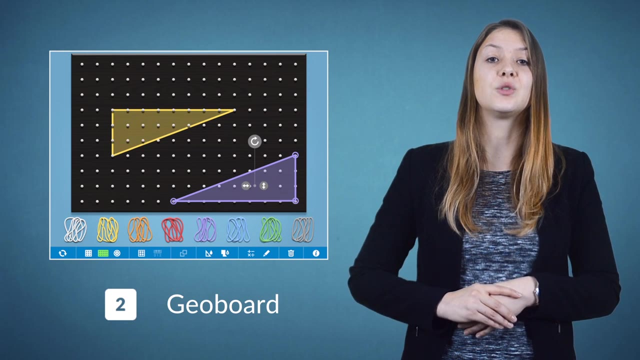 quiz-like lesson. The second app is GeoBoard. GeoBoard is a tool for exploring a variety of mathematical topics introduced in the elementary and middle grades. Learners must stretch bands around the pegs to form line segments and polygons to learn about area angles, fractions. 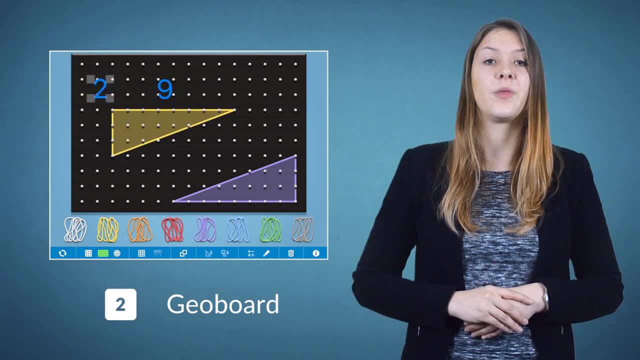 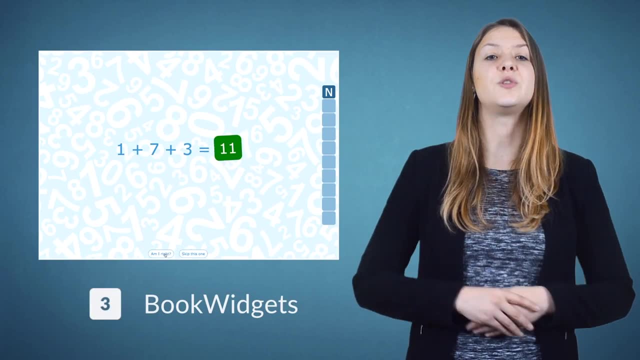 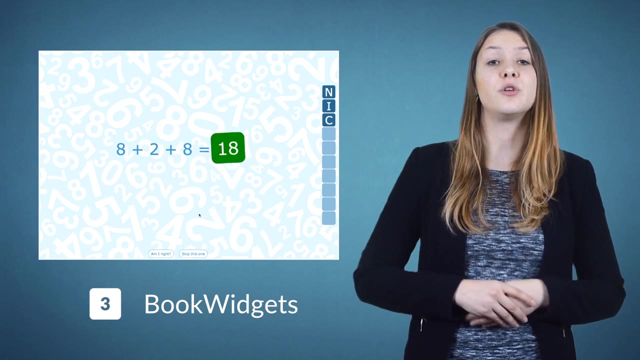 and more. It's an open-ended educational tool, ideal for elementary classrooms and other learning environments that use iPads. You can also use book widgets for teaching math. The youngest math pupils start by learning simple additions and subtractions, then move on to multiplication and division. The arithmetic widget lets them solve simple arithmetic problems. 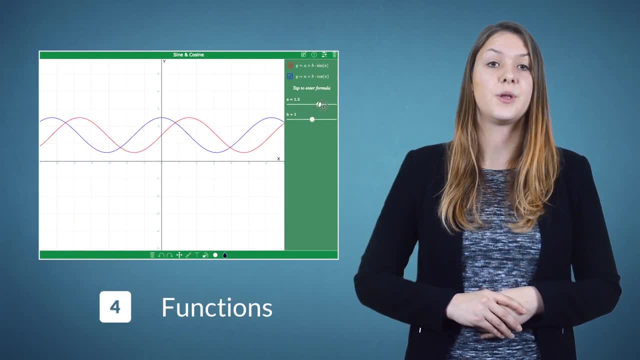 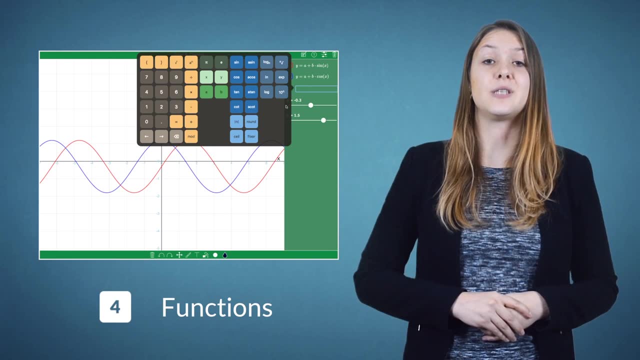 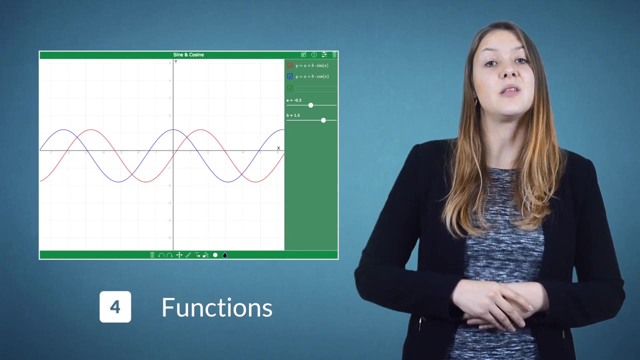 adapt it to their level. A lot in math involves functions. Knowing what these functions look like and how they change when their parameters change is key to understanding them. Creating your own interactive plot with the active plot widget is easy. Simply enter the functions you want your students to learn about and let them play with the parameters. Students. 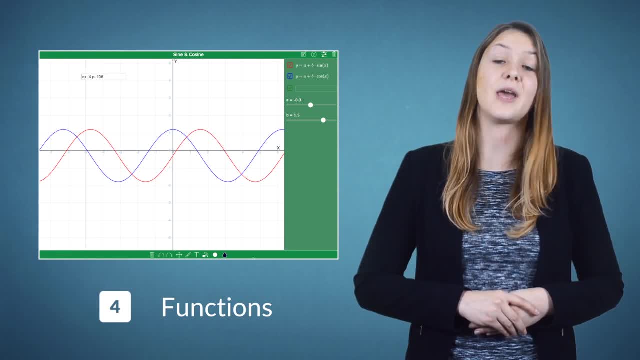 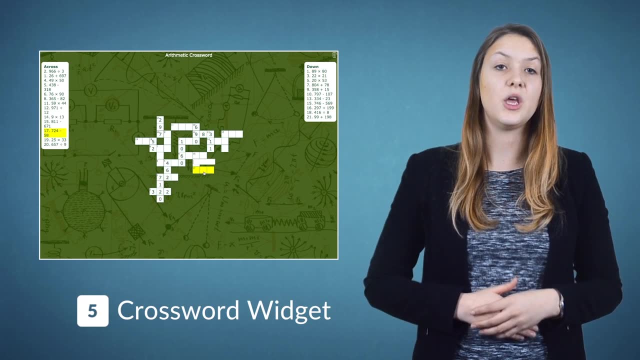 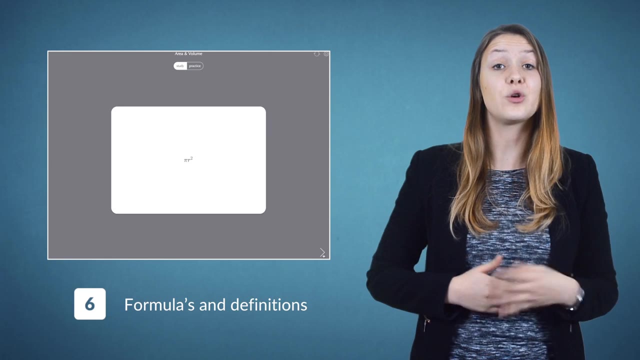 can also enter their own functions or using drawing tools to annotate the plot. The crossbar widget is a fun way to practice math terminology and definitions. You enter a definition and students fill in the words. Formulas and definitions need to be memorized. and the flashcard widget. 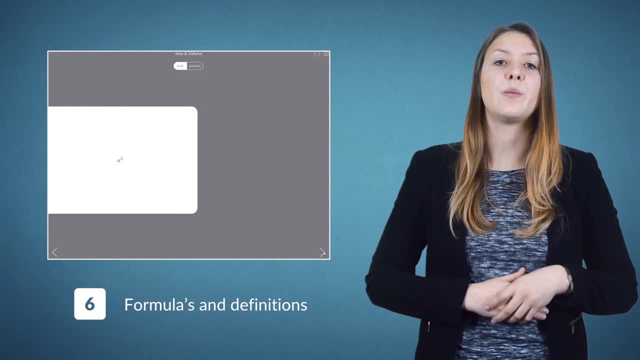 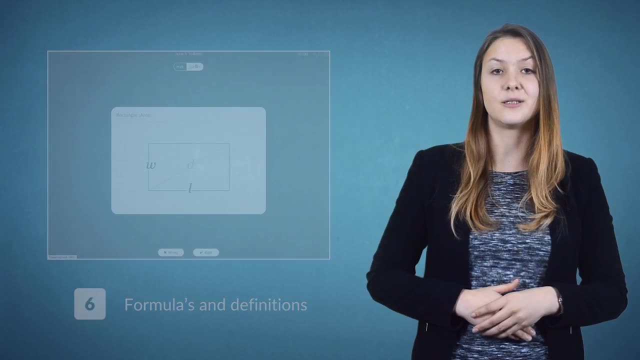 is a fun way to do so. For example, you can put pictures of geometrical shapes on one side and enter the formula to compute their area on the other side. Another fun way to practice math is by turning it into a pair matching game where students have to find. 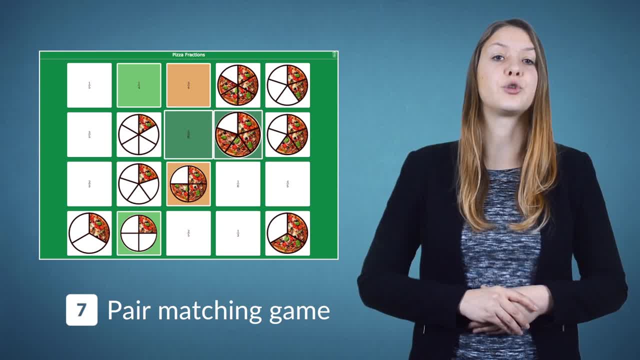 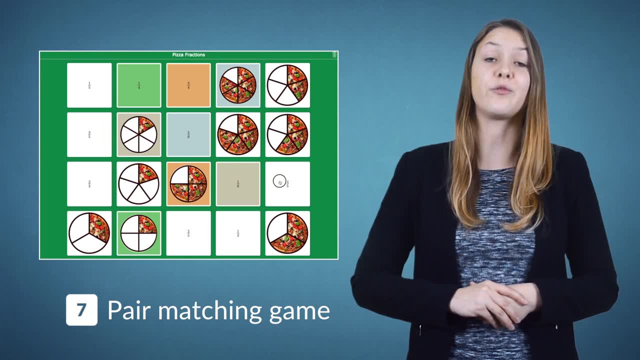 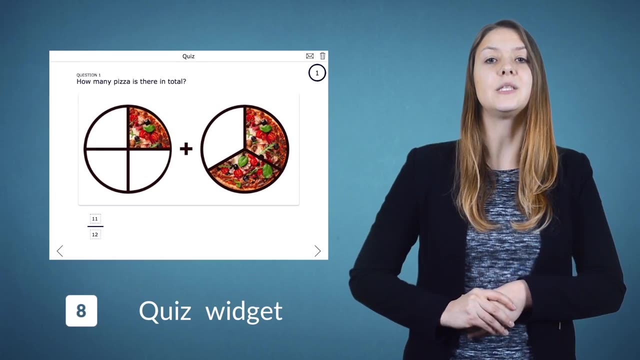 matching cards. You can create card pairs for terms and their definitions, equations and their answers. The younger pupils can play pair matching games to learn fractions. When they're done studying math, the time has come to test their knowledge. The quiz widget lets you do just.